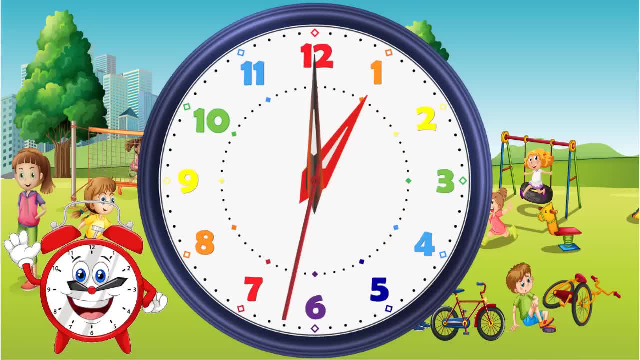 For this lesson, the second hand is not needed, Because telling the time doesn't require the telling of how many seconds have passed, Hehe, So let's take it off for now, Okay, So let's start with the hour hand. 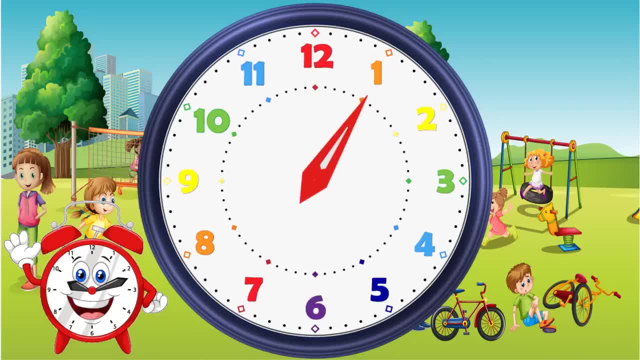 This will indicate what hour we are in. For example, This is one o'clock, Two o'clock, Three o'clock, Four o'clock, Five o'clock, Six o'clock, And so on, If the hour is in between the two numbers, as shown. 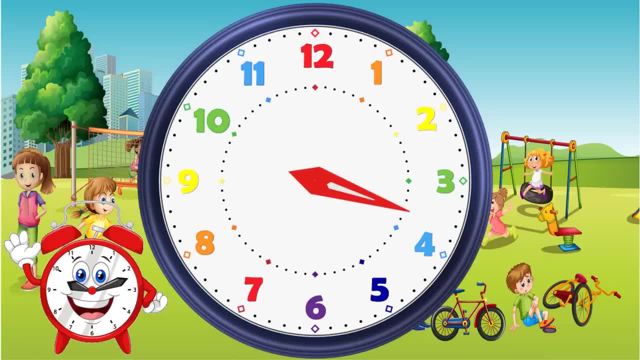 We will say it's in the three o'clock range. We'll explain this shortly. Now we have the minute hand. This indicates each minute that passes within the hour. So this is One minute, Two minutes, Three minutes, Four minutes. 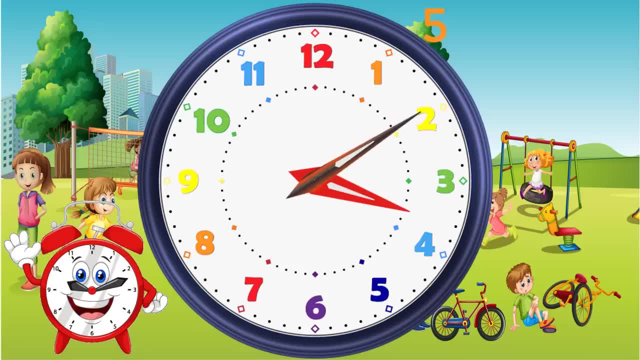 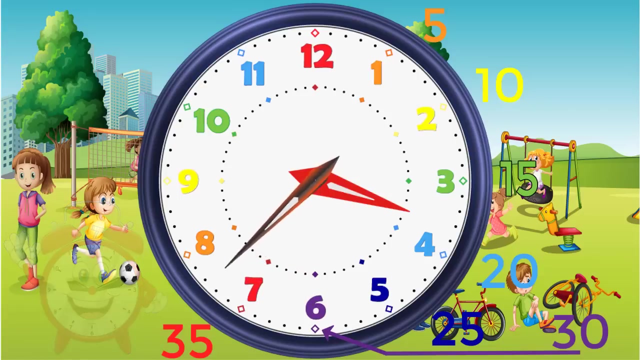 Five minutes, Ten minutes, Fifteen minutes, Twenty minutes. Twenty-five minutes, Thirty minutes. Thirty-five minutes. Forty minutes, Forty-five minutes, Fifty minutes, Fifty-five minutes And sixty minutes, So Sixty minutes to one hour. 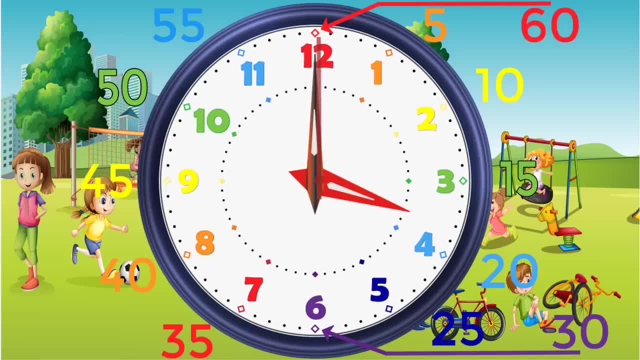 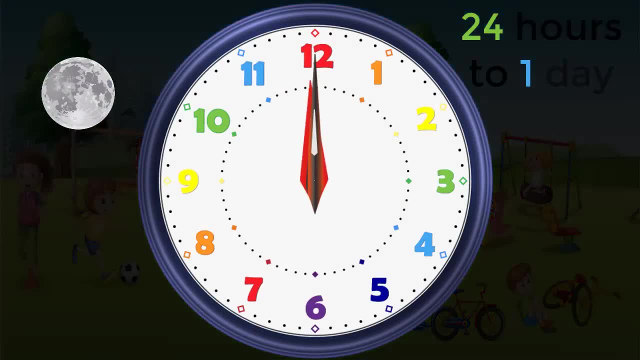 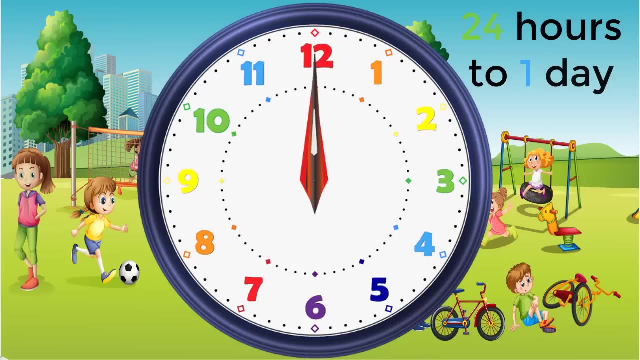 Sixty seconds to one minute. There is twenty-four hours to one day, Twelve o'clock at night to twelve o'clock midday, Then back to twelve o'clock at night. Twelve plus twelve equals twenty-four, So you can have a seven o'clock in the morning and a seven o'clock at night. 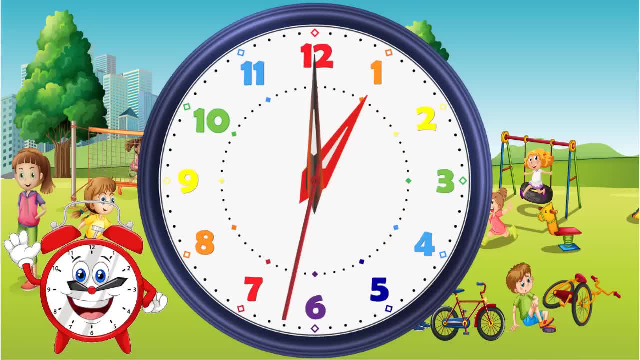 For this lesson, the second hand is not needed, Because telling the time doesn't require the telling of how many seconds have passed, Hehe, So let's take it off for now, Okay, So let's start with the hour hand. 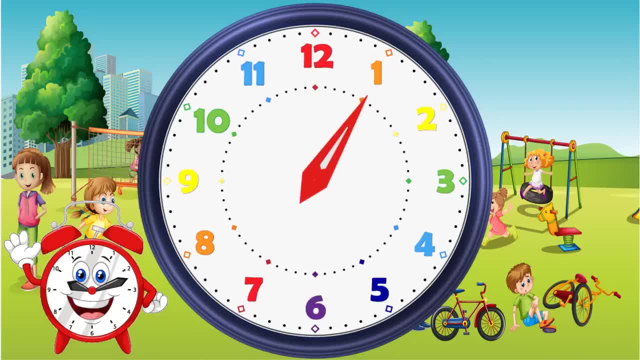 This will indicate what hour we are in. For example, This is one o'clock, Two o'clock, Three o'clock, Four o'clock, Five o'clock, Six o'clock, And so on, If the hour is in between the two numbers, as shown. 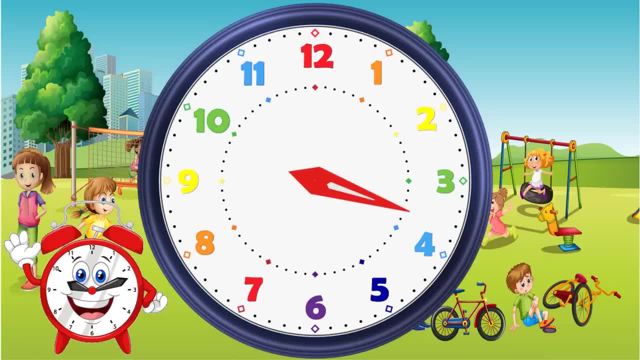 We will say it's in the three o'clock range. We'll explain this shortly. Now we have the minute hand. This indicates each minute that passes within the hour. So this is One minute, Two minutes, Three minutes, Four minutes. 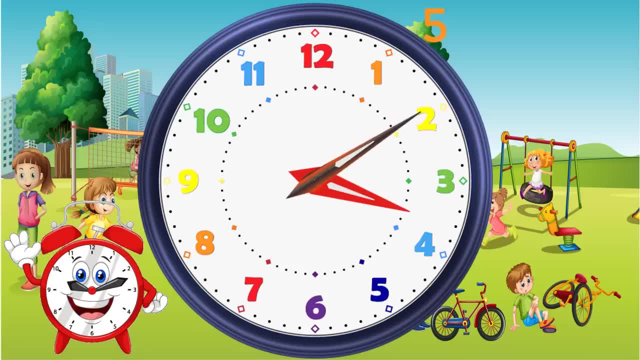 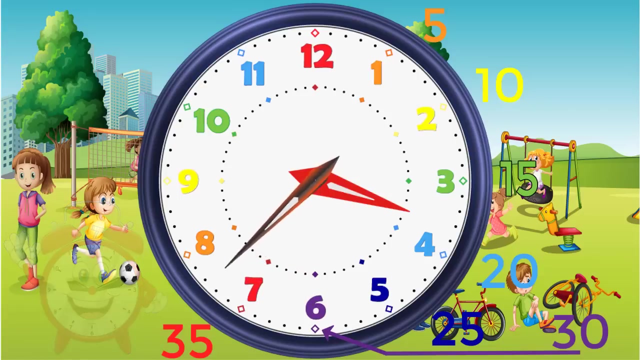 Five minutes, Ten minutes, Fifteen minutes, Twenty minutes. Twenty-five minutes, Thirty minutes. Thirty-five minutes. Forty minutes, Forty-five minutes, Fifty minutes, Fifty-five minutes And sixty minutes, So Sixty minutes to one hour. 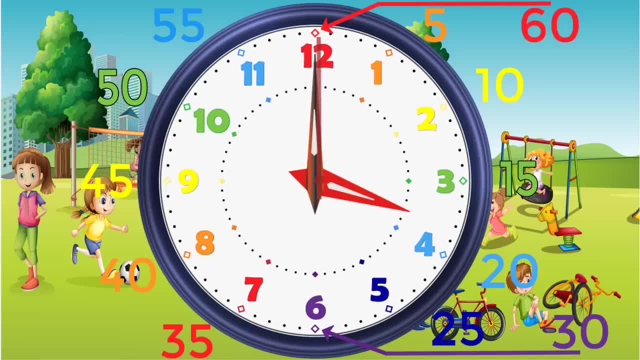 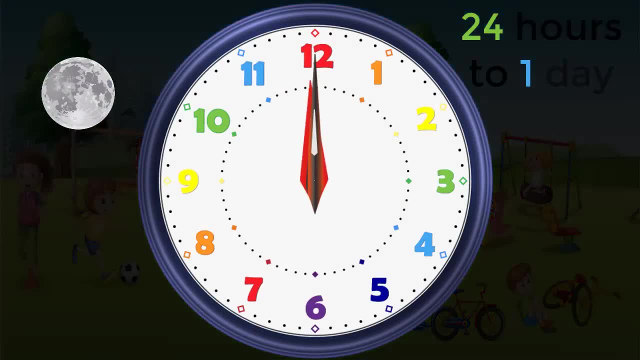 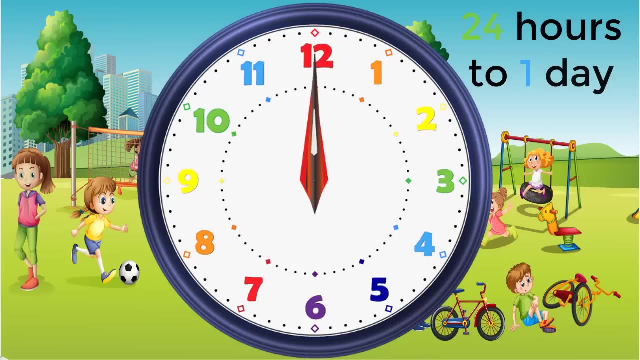 Sixty seconds to one minute. There is twenty-four hours to one day, Twelve o'clock at night to twelve o'clock midday, Then back to twelve o'clock at night. Twelve plus twelve equals twenty-four, So you can have a seven o'clock in the morning and a seven o'clock at night. 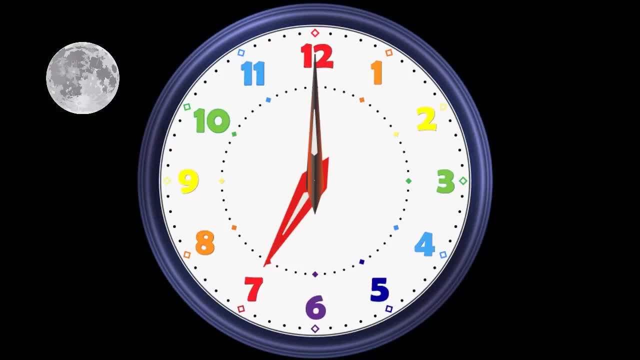 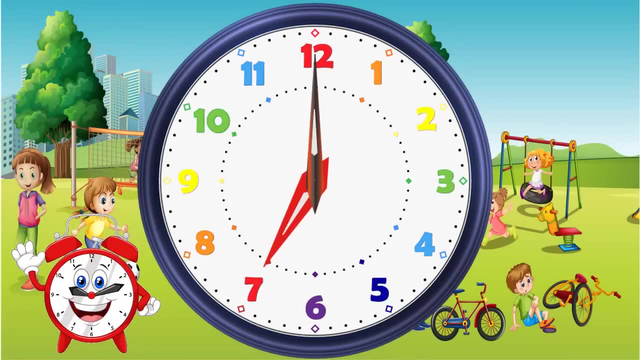 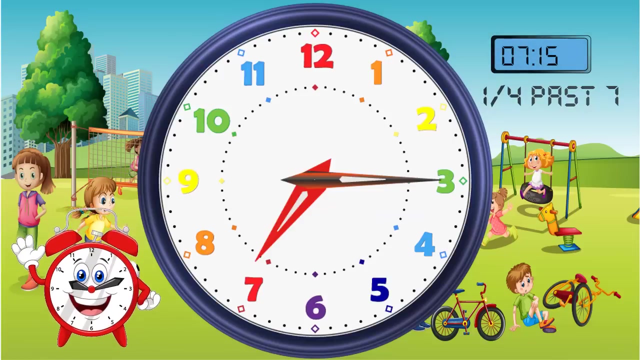 I'm so sleepy. So let's look at an important part of telling the time. When the time shows this, you can say seven-fifteen or quarter past seven, Because there is four quarters on this clock face: One, two, three, four. 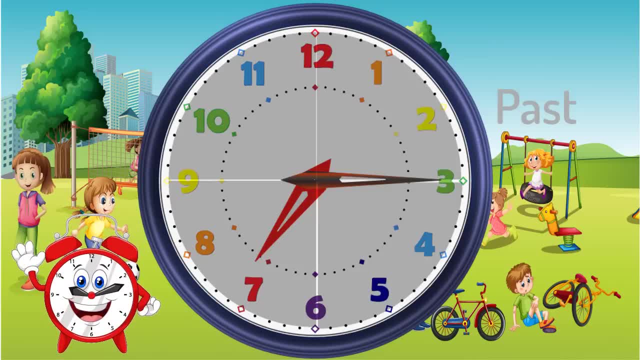 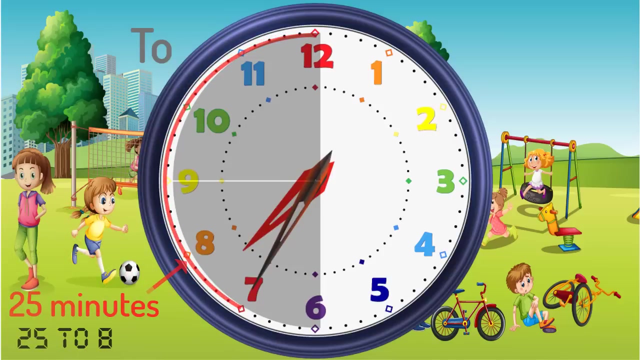 When using the word past, it's always when the minute hand is in this section of a clock face. When it goes past the six or the thirty-minute mark, we say two. The time showing now we say twenty-five minutes to eight. 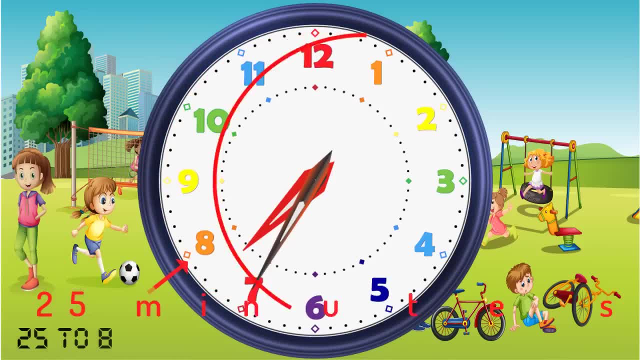 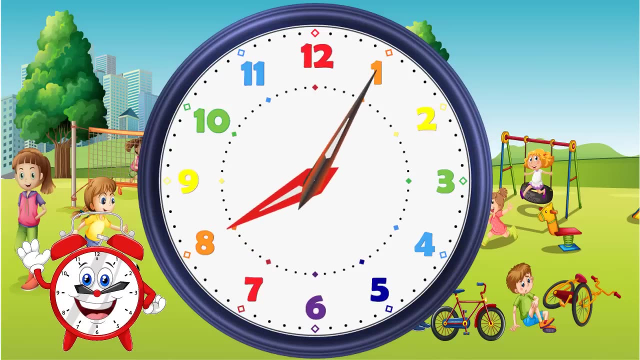 Or we can say seven-thirty-five, Because the minute hand is thirty-five minutes into the hour of seven. Let's look at some more samples. When we show this time it's eight-oh-five Or five past eight. 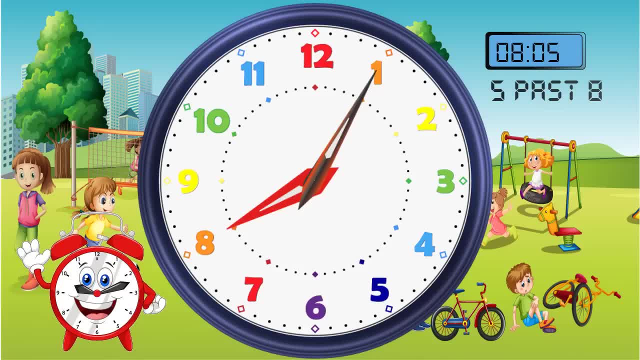 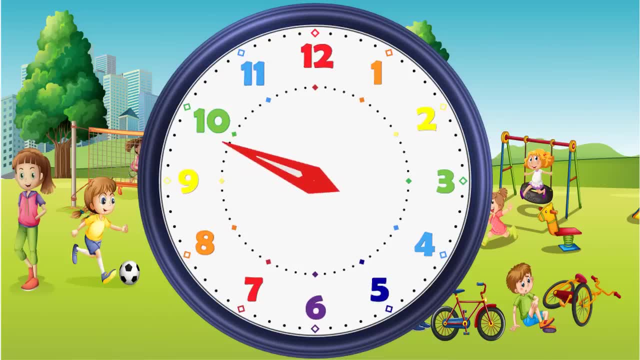 Think of all the numbers on the clock face as just numbers for the short hand. They are all numbers for what hour it is. Now there is also these numbers Used for the minute hand or long hand, So we can come up with the current time. 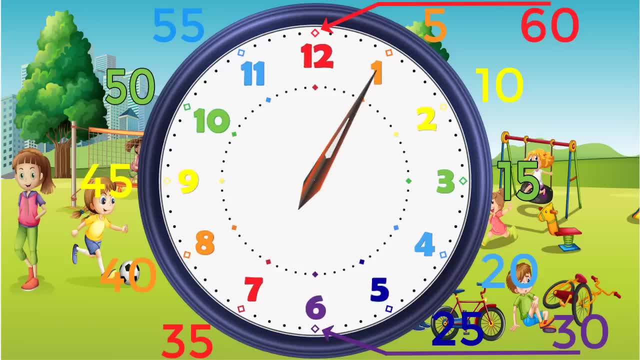 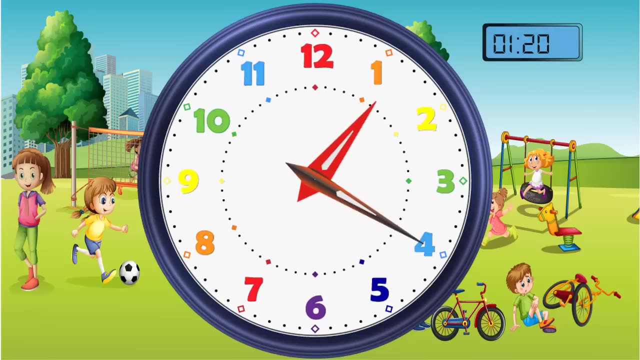 These numbers will get easier to remember the more you start telling time. Okay, so let's run through some times. This is one-twenty Or twenty past one. Now we have three-forty-five, Or quarter to four. 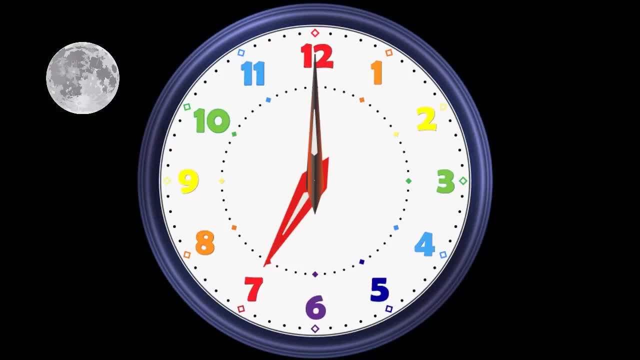 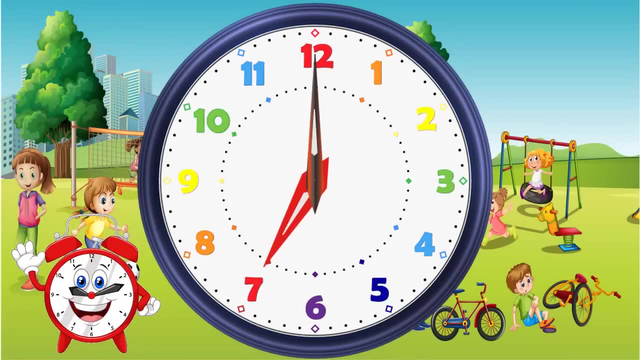 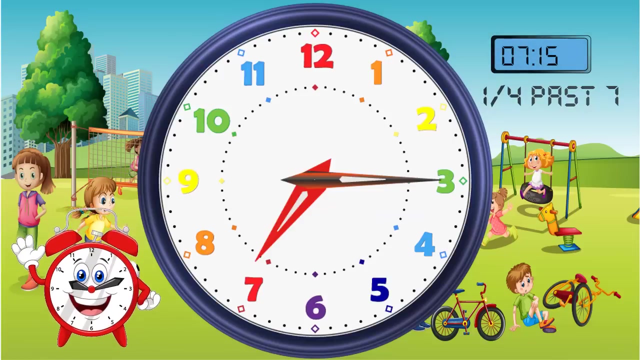 I'm so sleepy. So let's look at an important part of telling the time. When the time shows this, you can say seven-fifteen or quarter past seven, Because there is four quarters on this clock face: One, two, three, four. 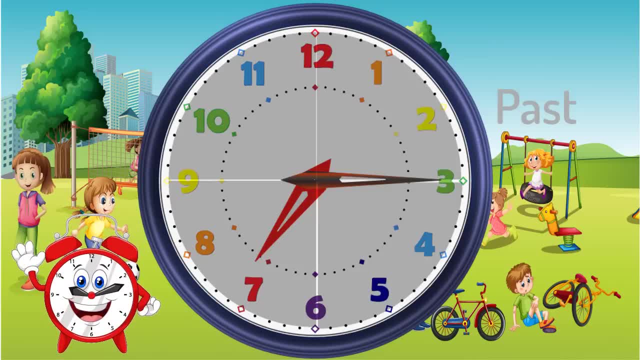 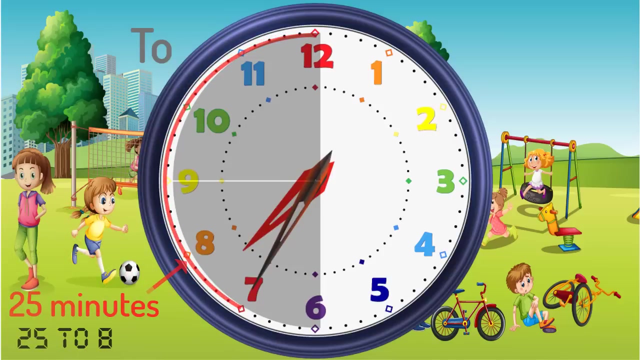 When using the word past, it's always when the minute hand is in this section of a clock face. When it goes past the six or the thirty-minute mark, we say two. The time showing now we say twenty-five minutes to eight. 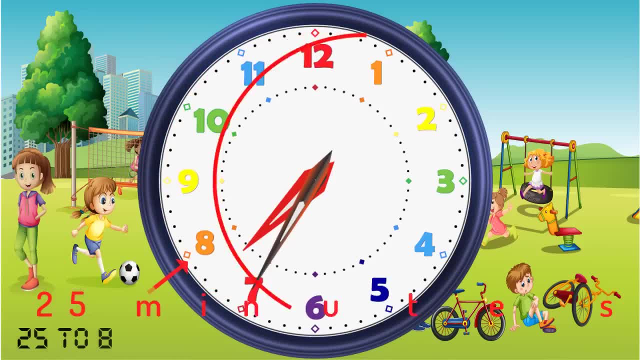 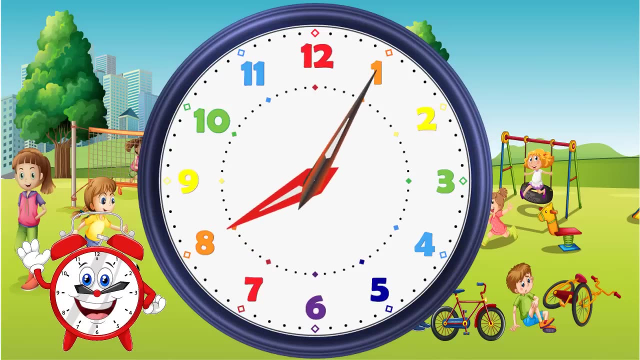 Or we can say seven-thirty-five, Because the minute hand is thirty-five minutes into the hour of seven. Let's look at some more samples. When we show this time it's eight-oh-five Or five past eight. 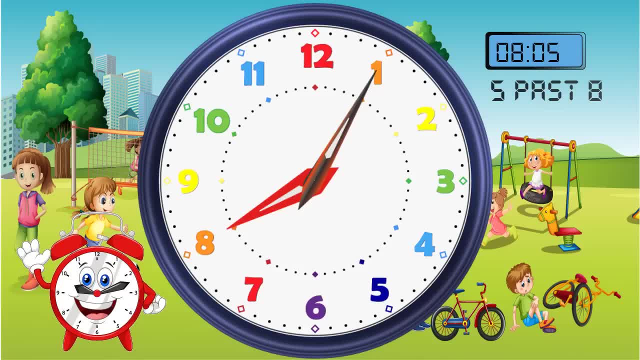 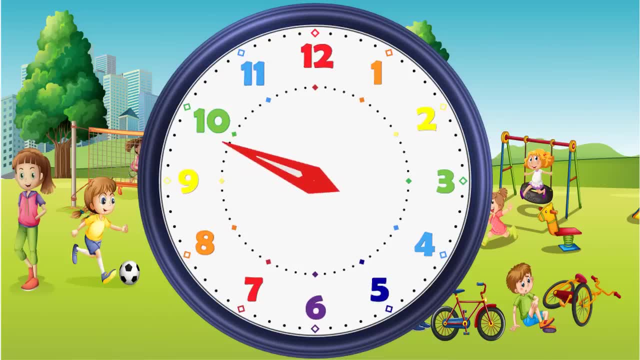 Think of all the numbers on the clock face as just numbers for the short hand. They are all numbers for what hour it is. Now there is also these numbers Used for the minute hand or long hand, So we can come up with the current time. 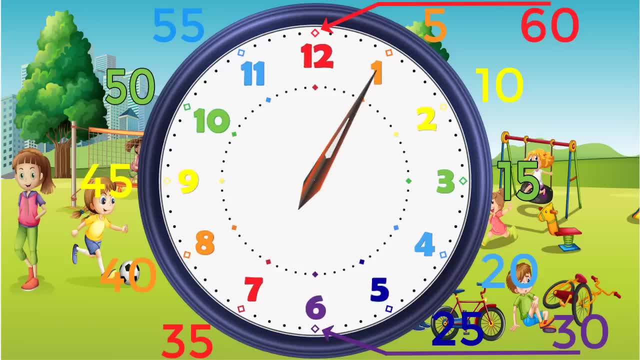 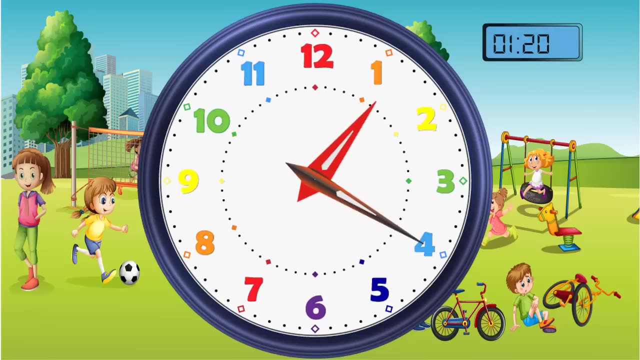 These numbers will get easier to remember the more you start telling time. Okay, so let's run through some times. This is one-twenty Or twenty past one. Now we have three-forty-five, Or quarter to four. 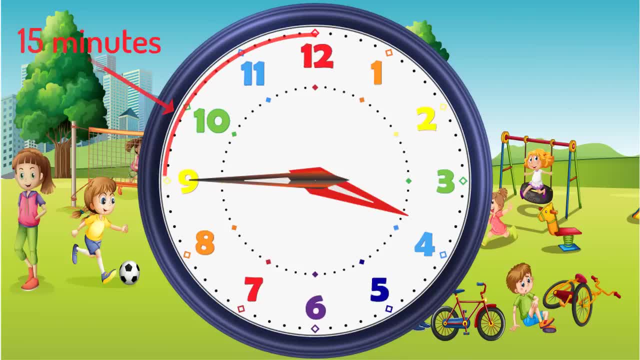 The quarter being fifteen minutes to four. Do you understand? Let's go through some more. This is four-fifty-five, Or five to five. In five minutes, the hour hand will be directly on the five Indicating five o'clock. 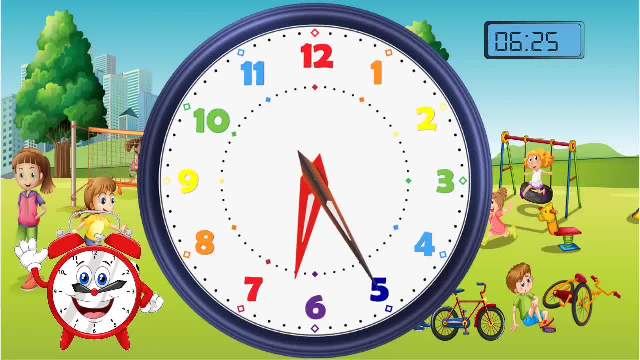 Now we have six-twenty-five, Or twenty-five past six. Here we have six-forty, Or twenty to seven. Okay, now it's your turn. I will give you some times, then we can have a try. 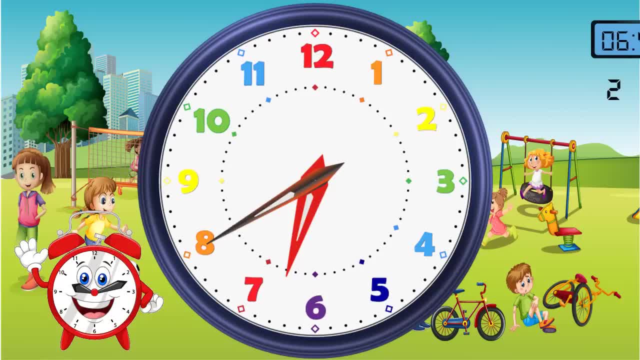 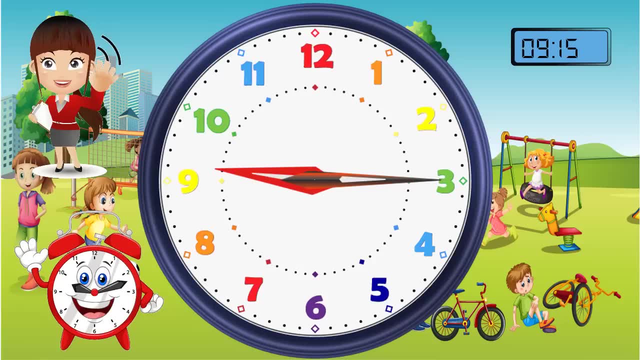 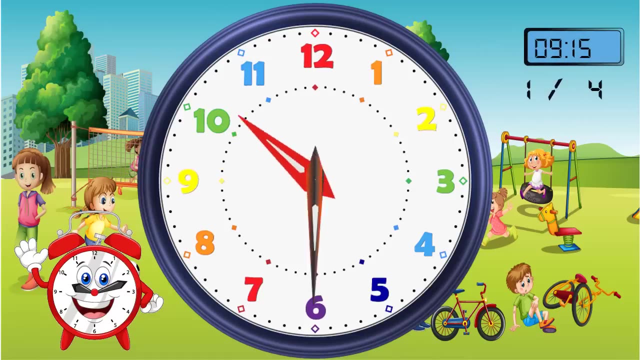 Then we'll see if your answer is right. What's this time? Did you say nine-fifteen Or quarter past nine? What's the time here? Did you say eleven-fifty Or ten to twelve? Okay, let's try a few more. 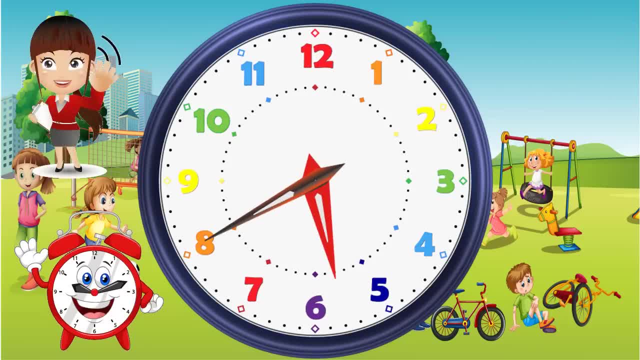 What's this time, Okay? Did you say five-forty Or twenty minutes to six? I hope you're going okay with your answers so far. Okay. What's this one? Did you say twenty past ten Or ten-twenty? 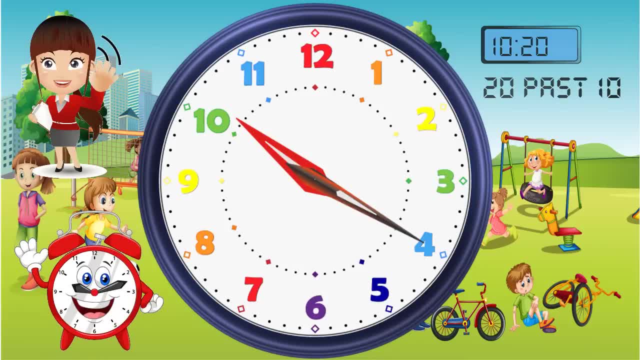 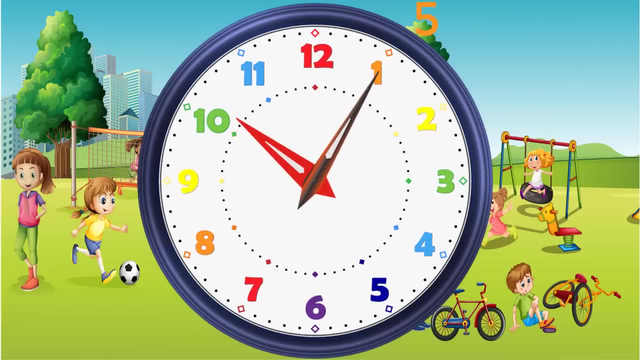 Very good, Just remember The minute hand. times is shown here. As a beginner, you can always count in fives to see how many minutes the long hand is on. So you can say Five, Ten, Fifteen, Twenty, That's twenty minutes past the hour of ten. 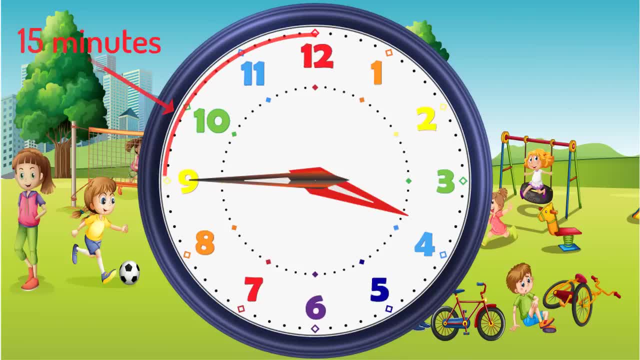 The quarter being fifteen minutes to four. Do you understand? Let's go through some more. This is four-fifty-five, Or five to five. In five minutes, the hour hand will be directly on the five Indicating five o'clock. 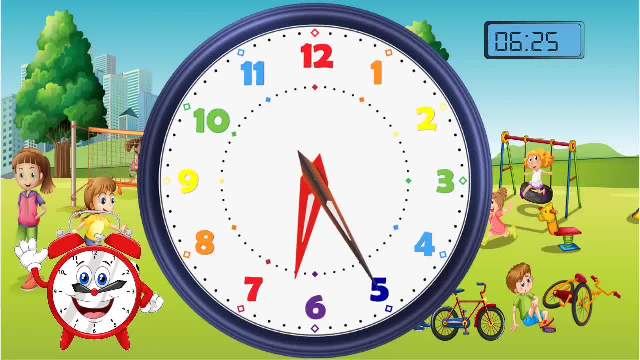 Now we have six-twenty-five, Or twenty-five past six. Here we have six-forty, Or twenty to seven. Okay, now it's your turn. I will give you some times, then we can have a try. 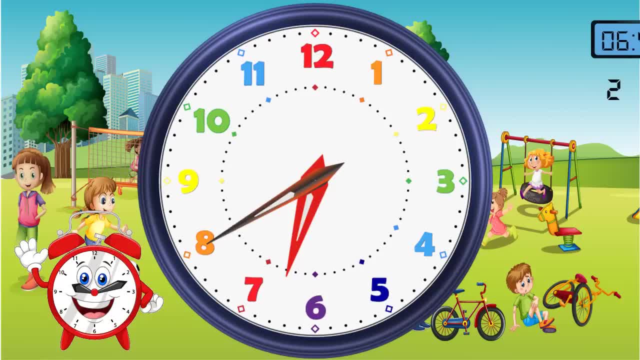 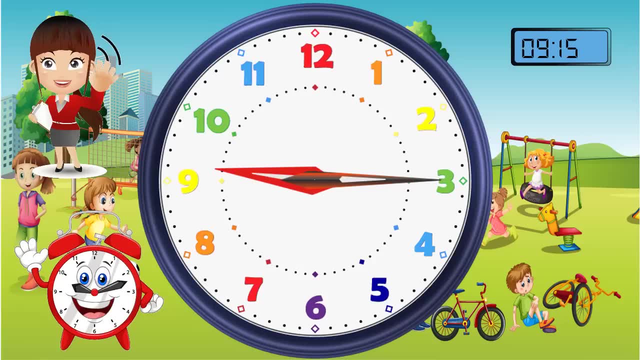 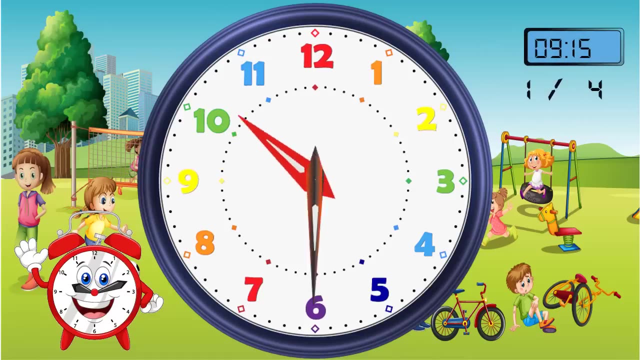 Then we'll see if your answer is right. What's this time? Did you say nine-fifteen Or quarter past nine? What's the time here? Did you say eleven-fifty Or ten to twelve? Okay, let's try a few more. 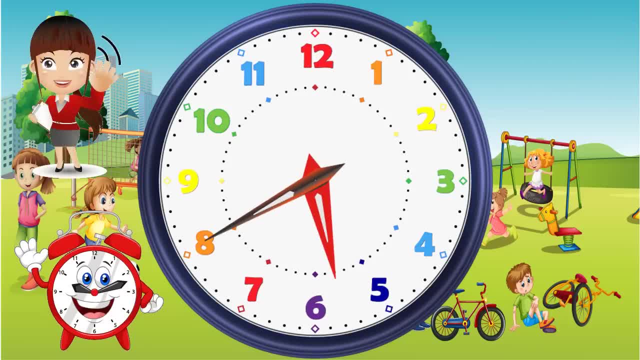 What's this time, Okay? Did you say five-forty Or twenty minutes to six? I hope you're going okay with your answers so far. Okay. What's this one? Did you say twenty past ten Or ten-twenty? 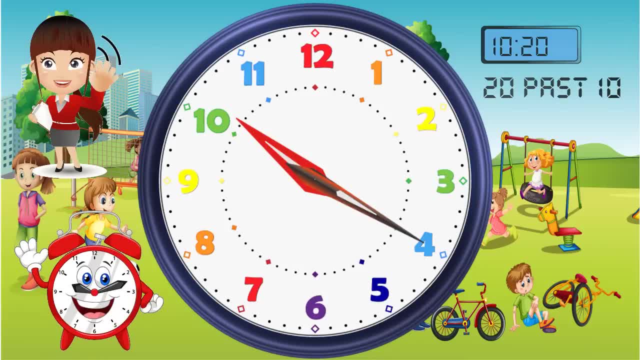 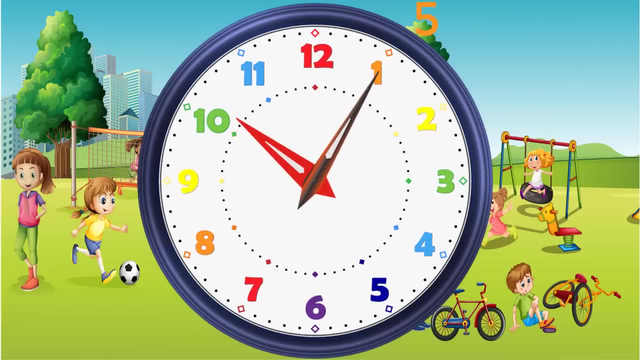 Very good, Just remember The minute hand. times is shown here. As a beginner, you can always count in fives to see how many minutes the long hand is on. So you can say Five, Ten, Fifteen, Twenty, That's twenty minutes past the hour of ten.